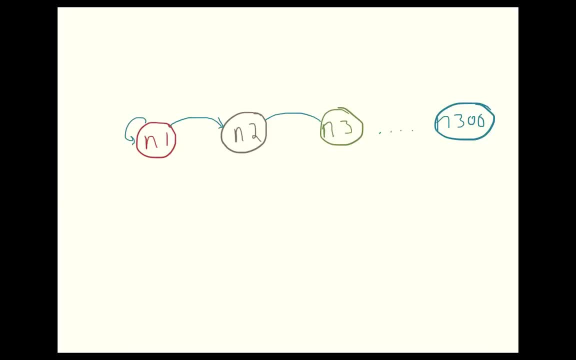 node is connected down the line. So it will work if we're looking at two nodes, but it would also work if we're looking and seeing if n1 was connected to n300.. So we'll take a look at how to implement that with some actual code here now. 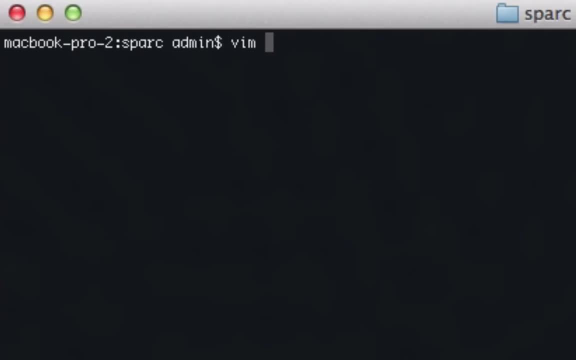 Okay, and we'll create our file. So we're going to call this one recursivespark And, first thing, set up our sorts, And we're only going to have one sort for this and we're going to call it node And set node equal to 1.4.. And now we'll do our predicates For 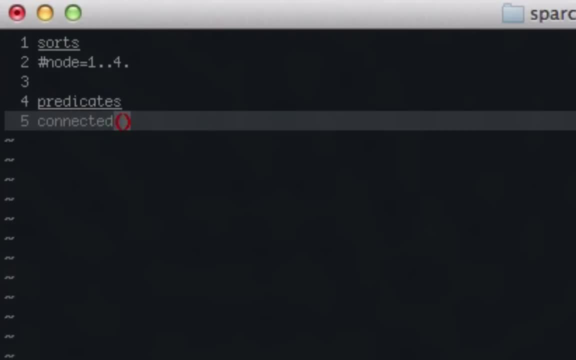 predicates. we're just going to have two. We're going to say connected node, node. So we're just saying a node is connected to another node And then we'll give another. you know type of connection where we say a node has an edge to another node. And if you think that 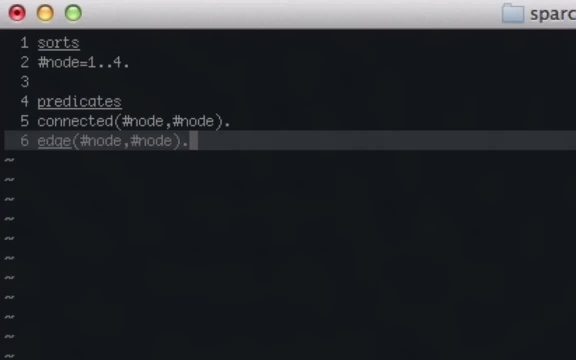 sounds like we're duplicating efforts. we're really not, Because connected means that if, say, node 1 and node 300 are not, they don't have an edge. So they're right, not right next to each other and they don't have an edge directly connected to them. However, if there is a direct 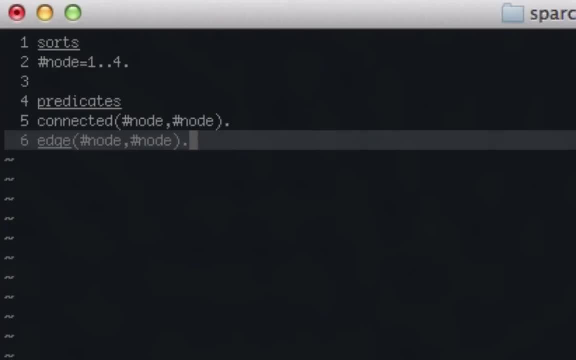 line that connects the every node between 1 and 300, then we would say that node 1 is connected to 300. But even though it doesn't have an edge, So we do have to put both rules in place to have this work. So now we'll set up our rules And I'm not going to set up all the 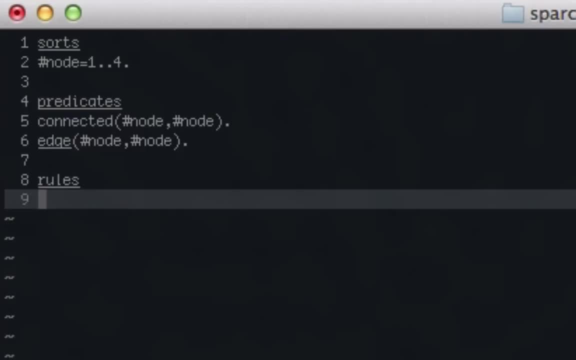 actual rules. So this is going to be a program that is a little bit more abstract. It's not going to put the details and let you know which node is connected to another node. It's going to give you all the details And then we're going to set up our rules And I'm going 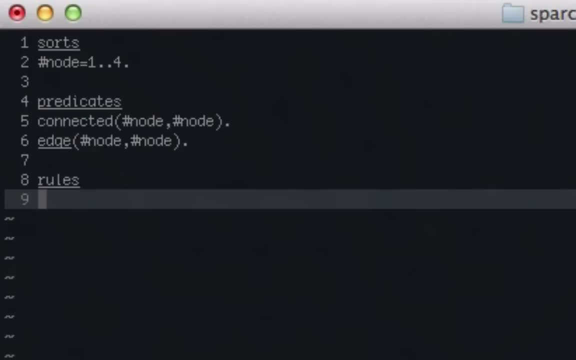 to put all the possible options, And it's just to show you how to implement recursion in a program. So the first thing is, when doing any kind of recursive function, is being able to establish a base case, And the very easiest base case is a node that is connected to itself. So 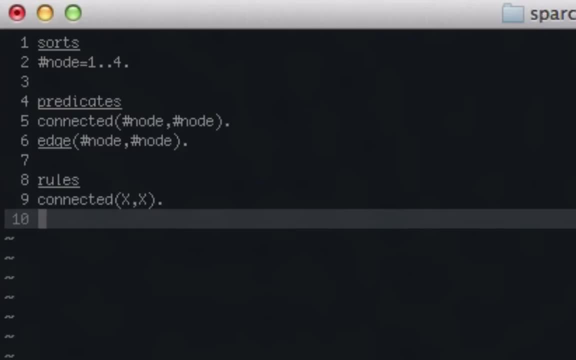 we're going to say x is connected to x. After that we're going to actually implement the real recursive call, And so we'll say x is connected to y if there is an edge that connects x to z and z is connected to y. And then 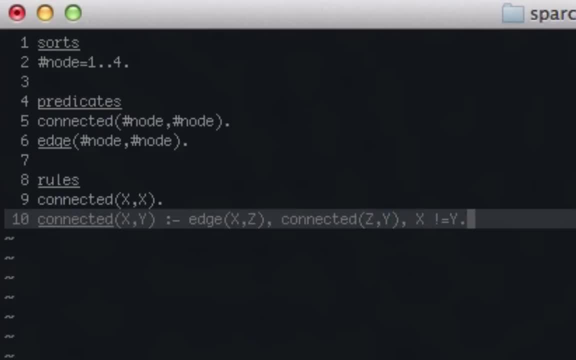 we'll make sure that x is not equal to y. The space isn't necessary, I just like it for reading. And then the last thing because we're going to set up our rules- is that we're going to set up our code to run something, because what this would do is it create some issues when we tried to actually 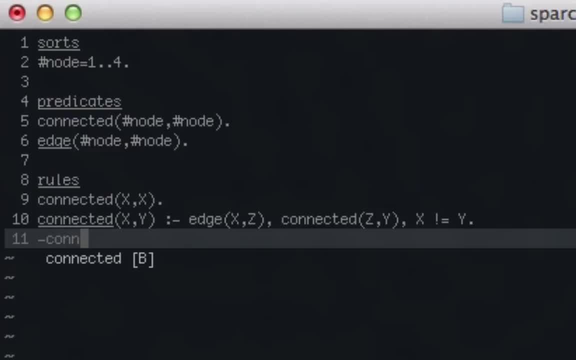 query the program. So we're going to say not connected. So we're going to say x isn't connected to y if there's no reason to believe, with default negation, that x is connected to y. So we'll save this and run it. I'm doing java, I'm going to do a little bit more of this code And it's running, And then we're going to set up our rule. So it's going to set up our rule. So we're going to set up our rule. 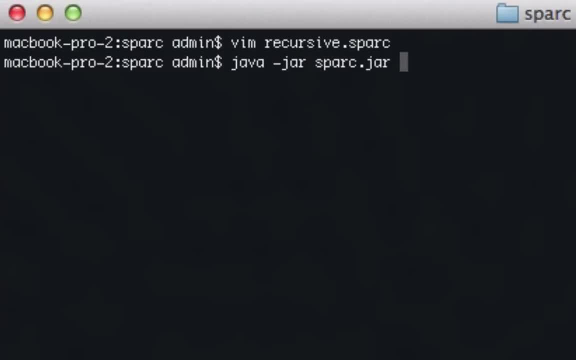 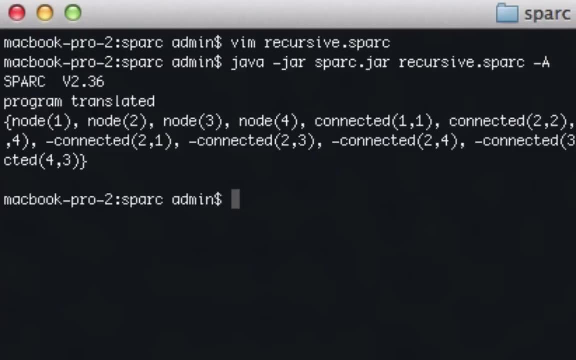 dash char spark, and we call this one recursive dash a, to see all the possible answer sets. and there you go, so you'll see that it goes through, iterates through the program, shows all of our nodes one through four, and then it shows all the potential connections. so it shows that you know. 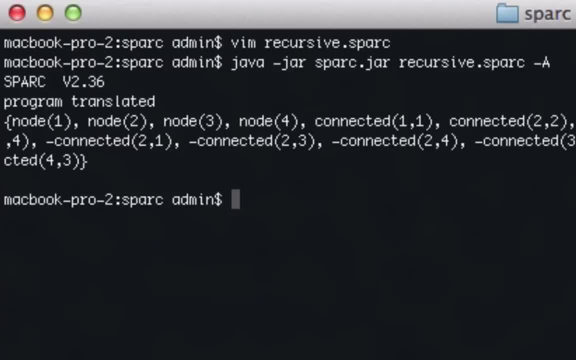 one is connected to one, two is connected to two and it's not showing that there are that any that are actually connected, because we didn't give any rules stating that. so if you want, you can go back in the program and say: you know, there's an edge between one and two and there's an edge between 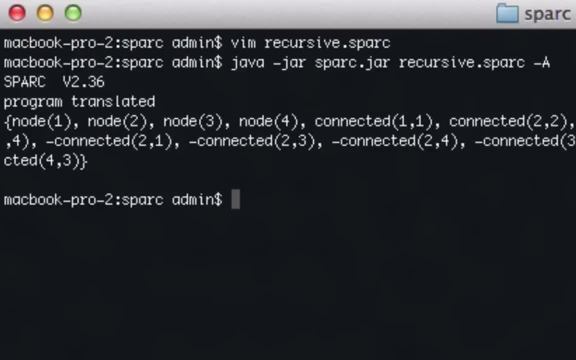 two and three and see that one and three are connected. but this is. I just want to show you the syntax for creating a recursive function. so if you went through that, congratulations, you know now. you now know how to do it. please let me know if you have any questions or if you can see any way that I could improve the program.